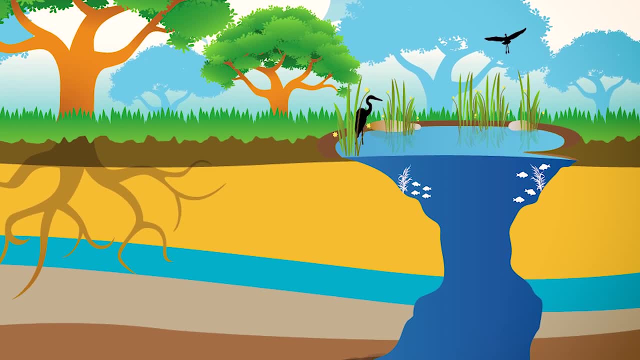 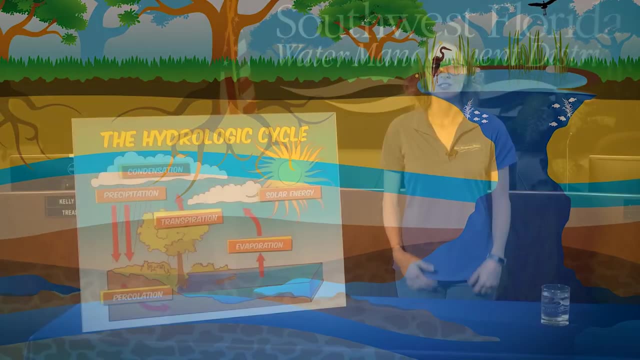 about 2 to 40 percent of the yearly rainfall that we receive will go down into the ground. That's why it's so important for us to be mindful of how much water we use every day. So where does our water go when it's not underground? Let's take a look. Water is constantly moving. 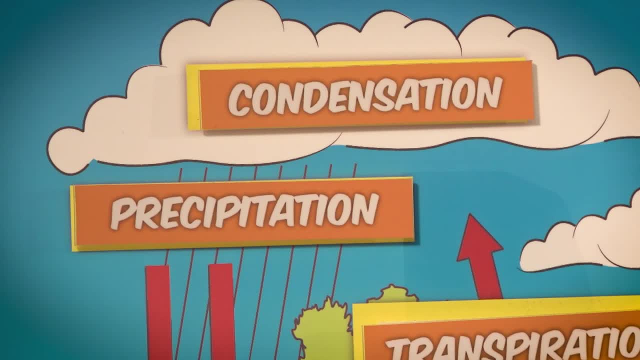 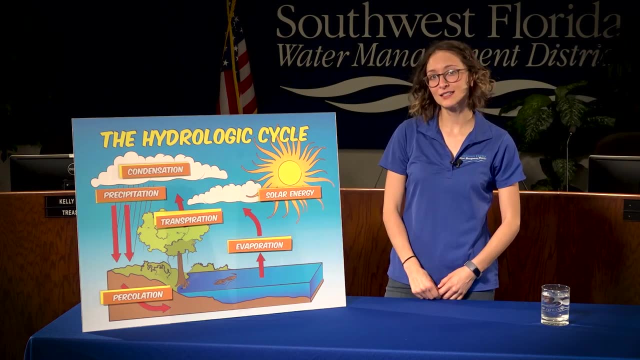 through what's called the water cycle. It might be floating in the clouds, chilling in a glacier, hanging out in the ocean or moving up through a plant. Since water is constantly moving, that means it's not always available to us Only about 1% of the water. 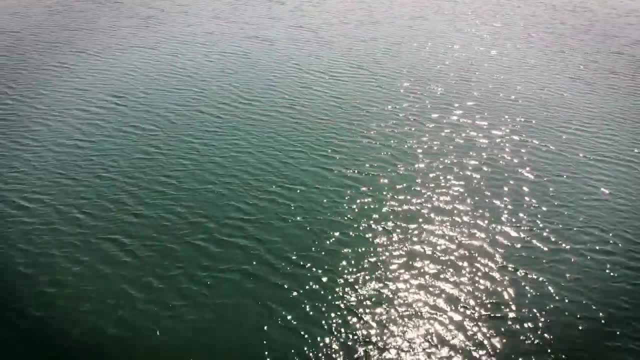 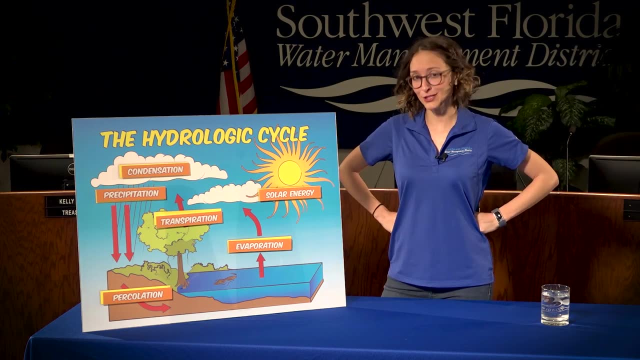 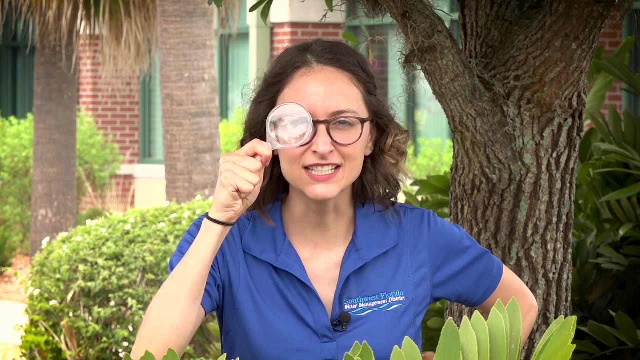 on Earth is fresh water. That's why it's so important for us to conserve. Now, what do you say? we find out a way that you can learn more about water right at home. We're going to become water investigators and try to find all the different ways we can see water and how it moves, right at our 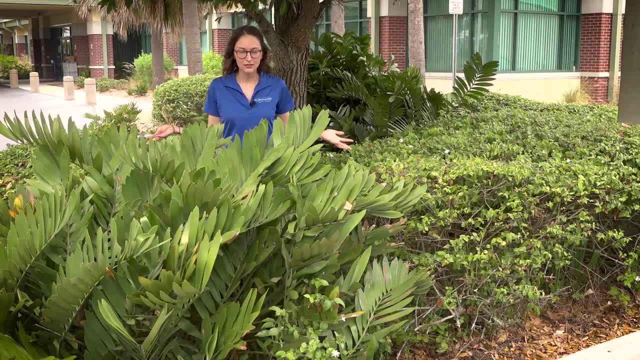 own homes. Let's start right here in your backyard. Now we talked about how you drink water. Is there anything else in your backyard that you can learn about? Well, we're going to start right here in your backyard. We're going to start right here in your backyard. 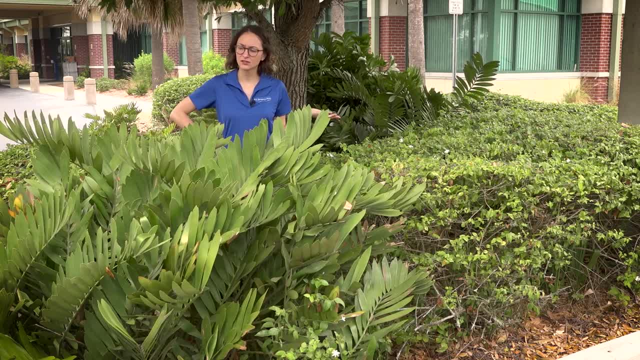 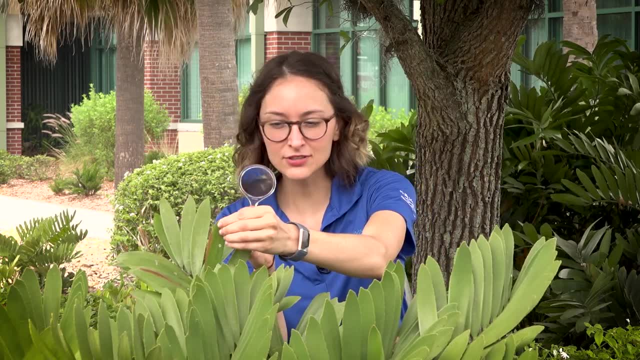 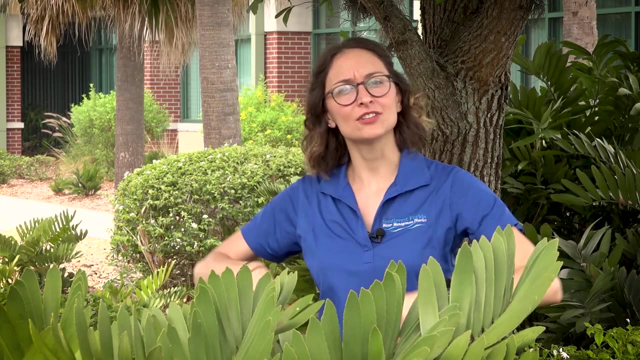 Is there anything else in your backyard that you can think might drink water too? Hey, I know Plants. Plants drink water up through their roots before entering out through their leaves. Plants sweat water just like we sweat through our pores. Where else do? 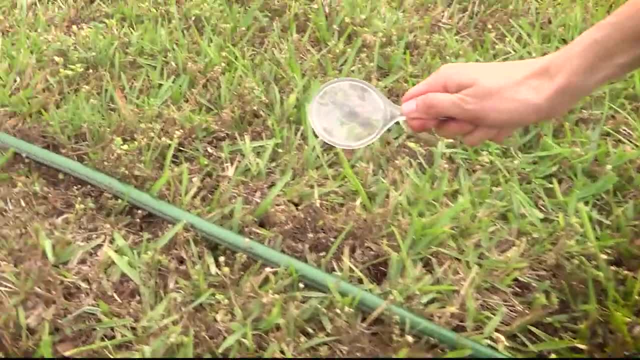 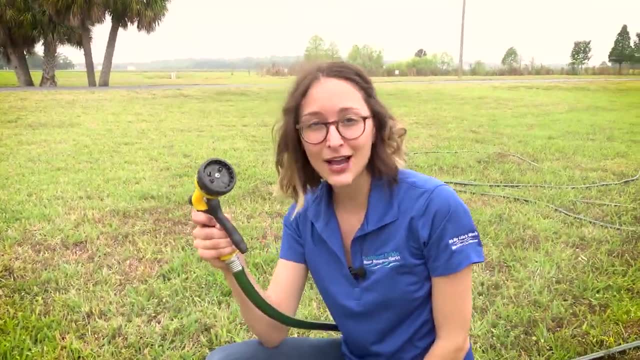 you think we might be able to find water outside. Now I bet we can find water here somewhere. Oh, A garden hose. Make sure if you have a garden hose you have a shut off hose. What's in your backyard? There's a hose to make sure you don't get wet. You can go to. 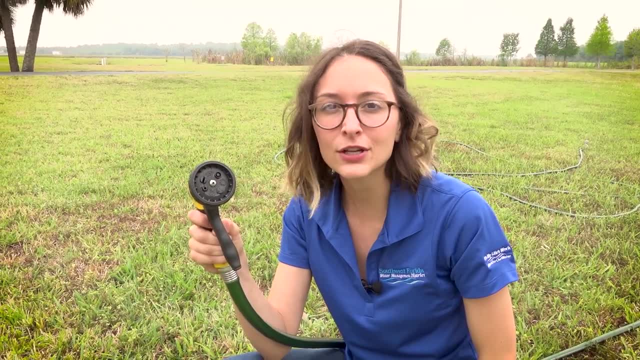 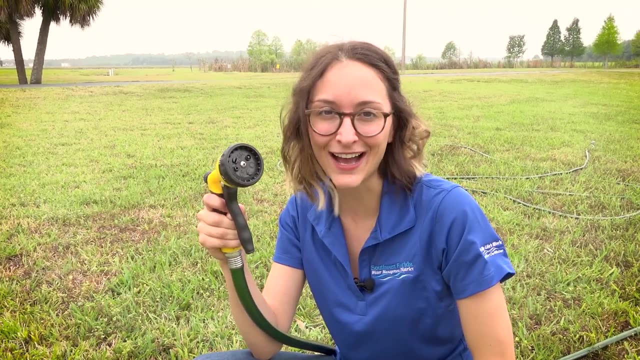 off nozzles so that water's not constantly flowing out. One of the most effective ways to save water at home is to conserve outdoors. Now let's go inside and see what we can find. Now that we're inside, let's try to find water. 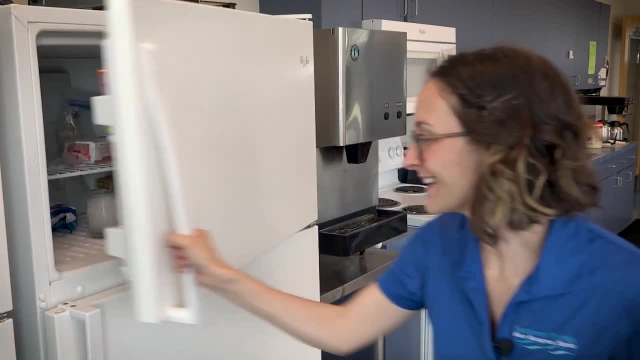 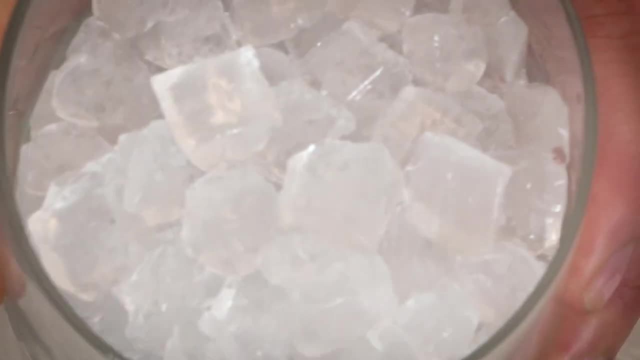 in a solid state. I know the freezer Ice is one of the many states that water takes as it moves through the water cycle. In fact, a lot of our fresh water is stuck in glaciers or ice caps. Now that we've explored around here,